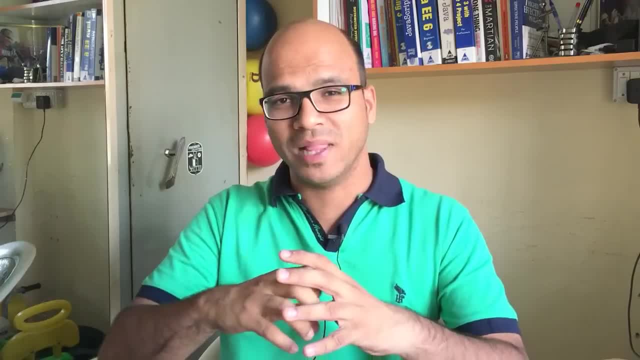 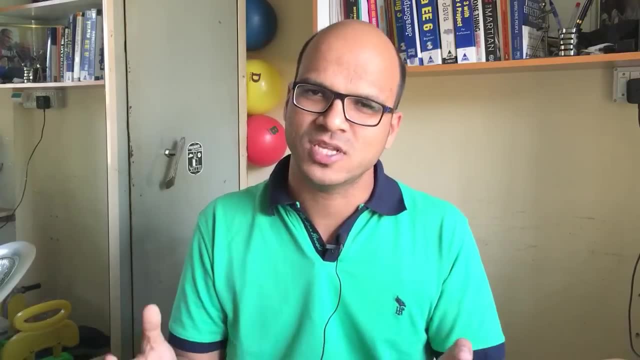 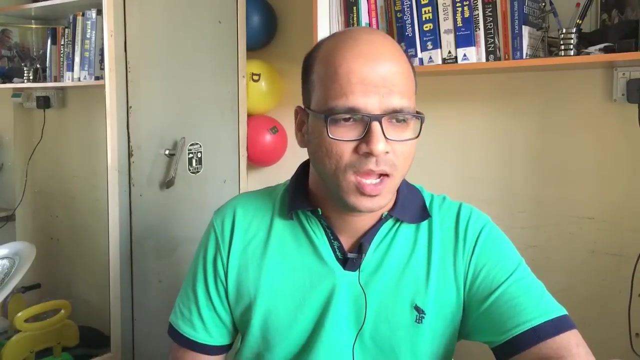 language which was built. I mean, the main motto of building a language for Scala was to make it scalable, and that's why Scala stands for scalable language, So name suggest that it is scalable. so, yes, it is one of the important feature of Scala. Now, what next? The world? 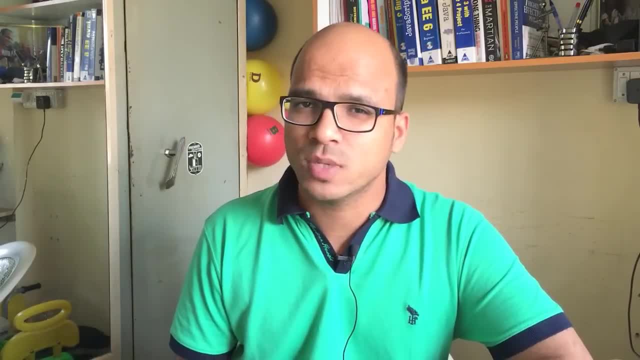 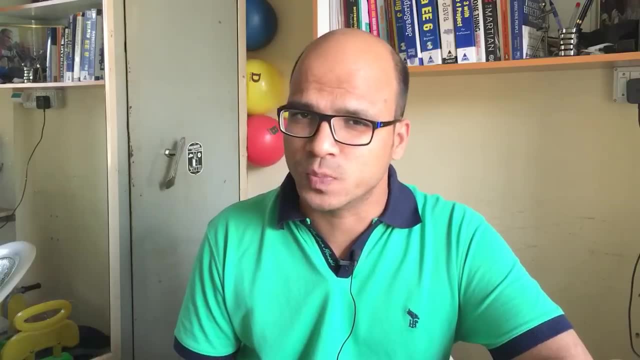 is changing right. in fact, everywhere we are generating huge amount of data. So we have this constant data. So we have this constant data, So we have this constant data. So we of big data and to work with big data, we need to work with a framework called as Hadoop. 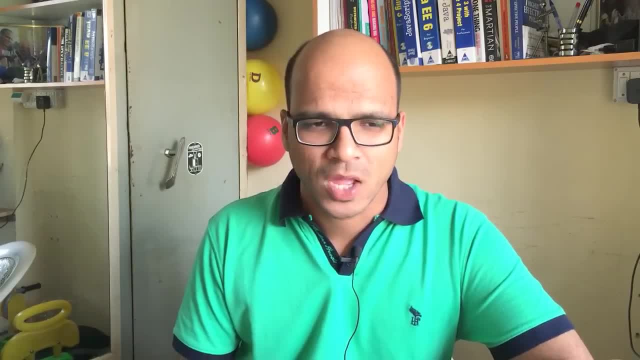 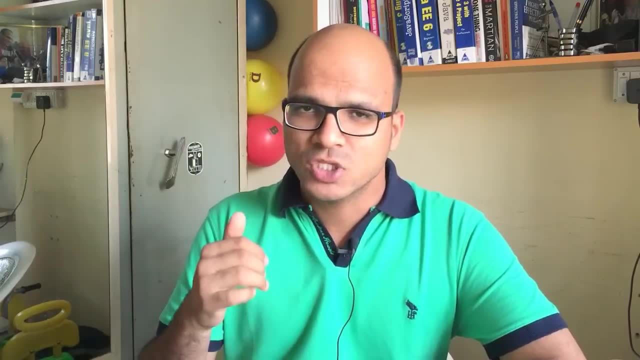 and so we have this framework, which is Hadoop, and we have one more which is the latest framework, for big data is called as Spark. so we have Hadoop and we have Spark. so if you work with Hadoop, we can use Java, we can use Scala, but if you work with Spark, the only language we 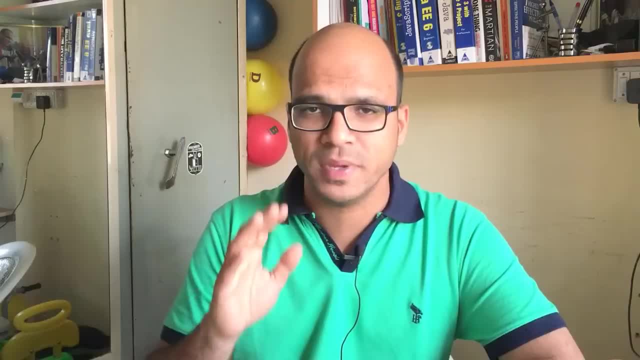 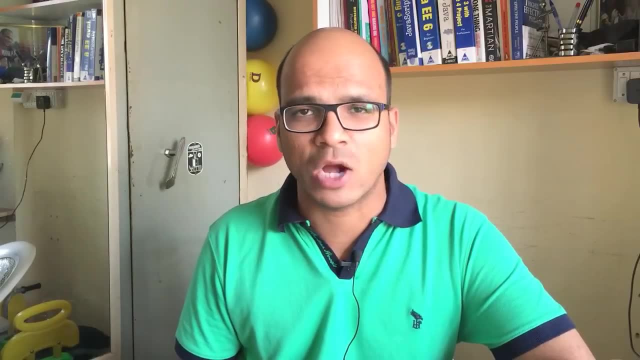 can work with is Scala. so, in case, if you are going for big data on Spark framework, you need to learn Scala. in fact, if you are, if you are going for the cloud data certification for Spark- I mean Hadoop Spark- we need to know Scala programming language. so it is very it's. 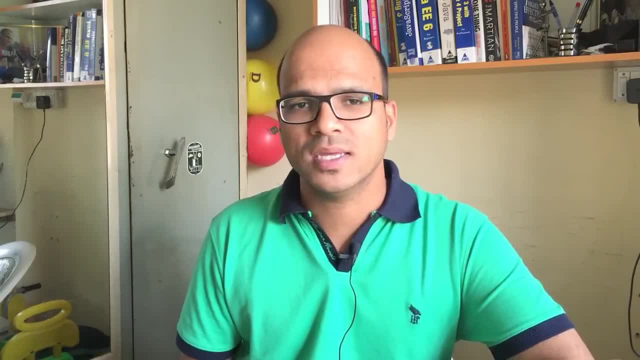 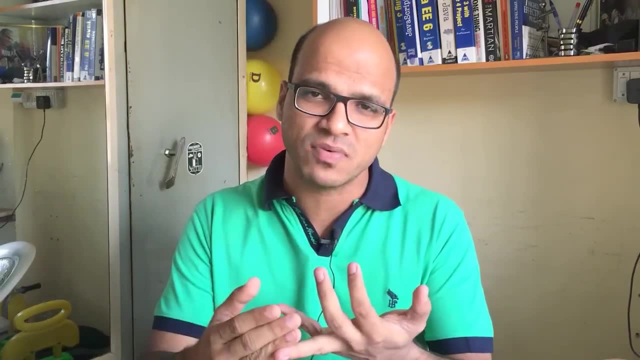 that important. next important thing is: you know, there are lots of people. they always debate with me about their favorite language. so they like Python, I like Java. so what happens is when I say Java is good, it has so many features, then this people who love, who loves. 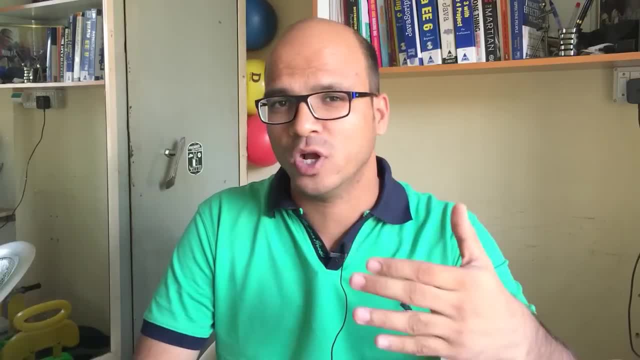 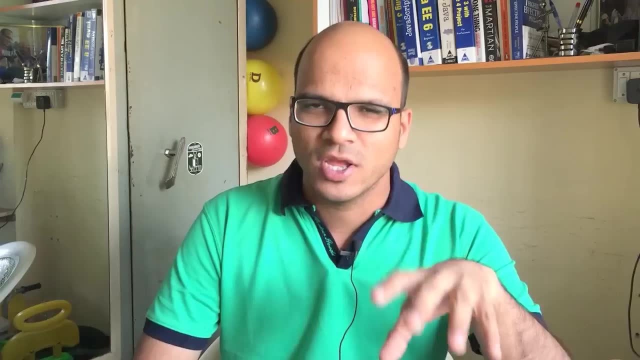 Python. they say: you know, in Python, when you want to play with Python, you want to play with print, hello world, we can write only one line, the same thing you can do in Java. you have to write approximately six lines of code. you have to create a class. you have to create. 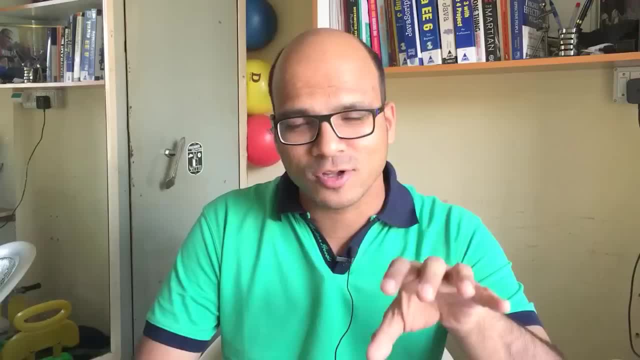 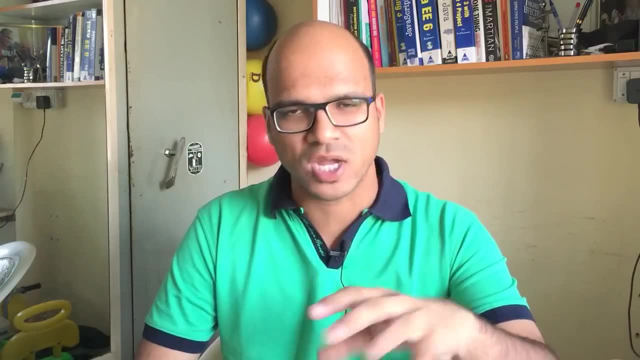 a main method. you have to create a system out dot println, then you can say: hello world, right. it's, it's bit odd, it's because in Java we have it is a structured language. I love Java, I mean. I mean you know about it, right, so I have a whole channel on Java. so but the thing, 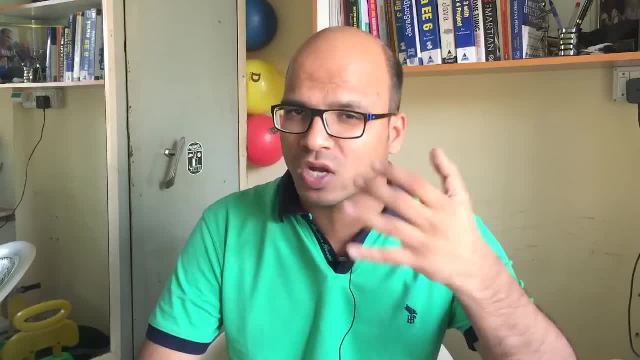 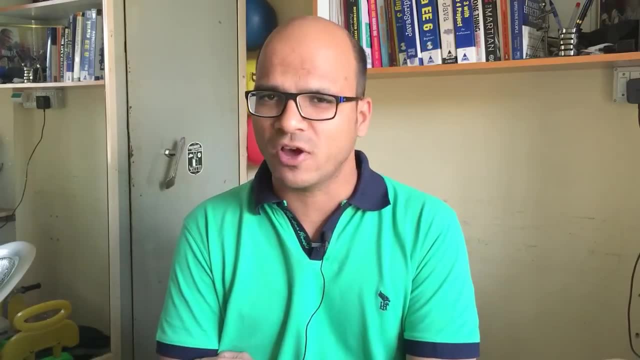 is yes, there is a boilerplate code in Java because it is more structured for Google, so it is more programming and so it has certain boilerplate codes. now Scala says: you know, there are lots of Java programmers. they think you know Java should be modified, we should. 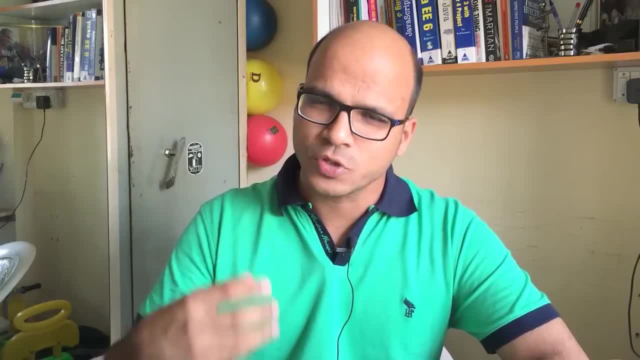 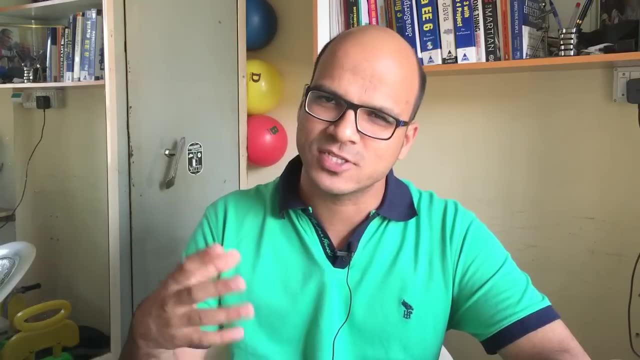 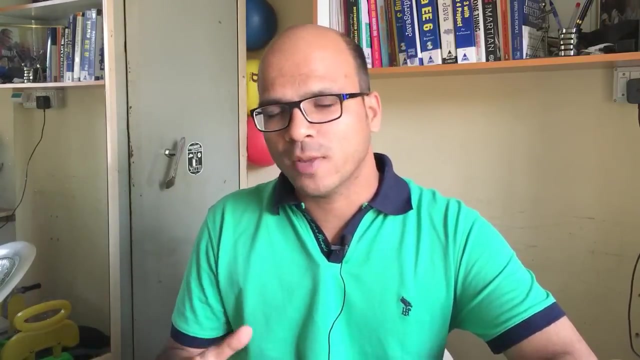 make it less boilerplate code. so they tried to modify Java and they came up with Scala. okay, so we cannot say Java. there is much difference between Scala and Java. it is, Scala is almost Java with some changes. I mean that sum is very important. okay, so there is no boilerplate. 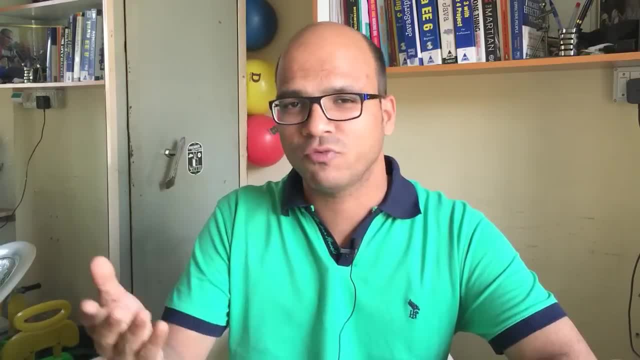 code in Scala, if you want to print something, you can directly write a line. you can print directly. write a line and it will print for you, so you don't have to write any boilerplate code there. when it comes to boilerplate code, it simply means you know those lines which. 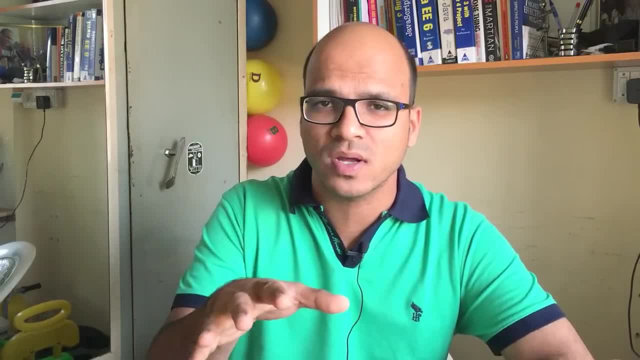 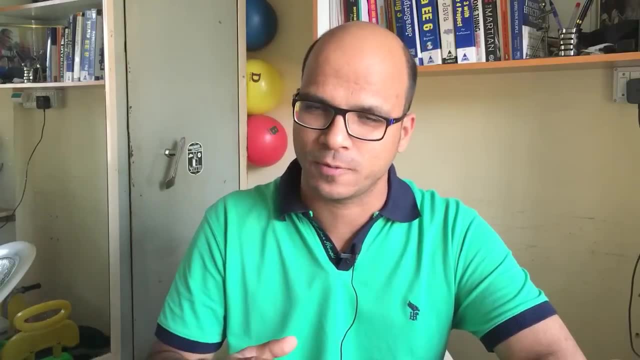 are not important. example: if you want to print hello world in Java, the most important line is system dot out, dot println. but still we have to write class. we have to mention the main method, that is, boilerplate code. what else Java supports concurrency? now why we need. concurrency is because we are living in an age of octa-core CPUs. so in our CPU, initially we used to have one core, and now we. then we got two cores, which is dual-core machines, then we got quad-core machine and now we have octa-core CPUs. so when you have octa-core CPU, 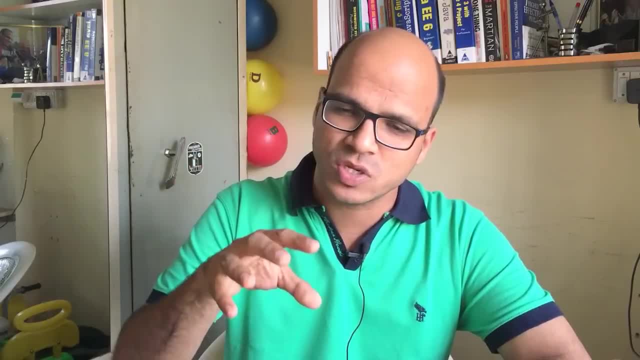 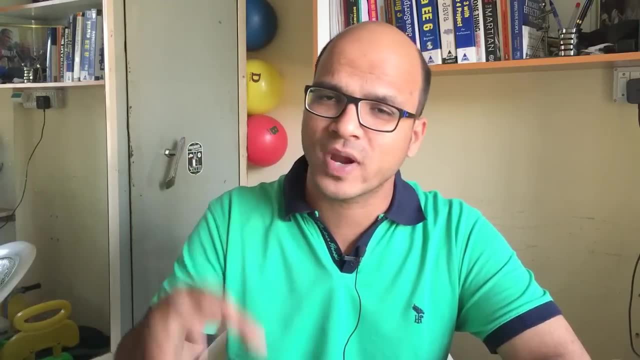 that means you have multiple cores. so we have to make sure that when you write a software, it should be that efficient that it will use all the available codes, and Scala provides you that feature. even if you don't know that you are doing it, Scala will do automatically. 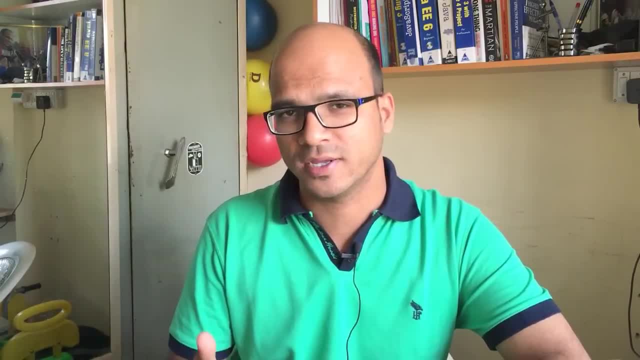 for you. so Scala provides concurrency. so we have talked about: Scala is similar to Java, but it is a little bit different than Scala. it is a little bit different, but it is a little bit different than Scala, because Scala is scalable language. it works on big data. it is. it doesn't. 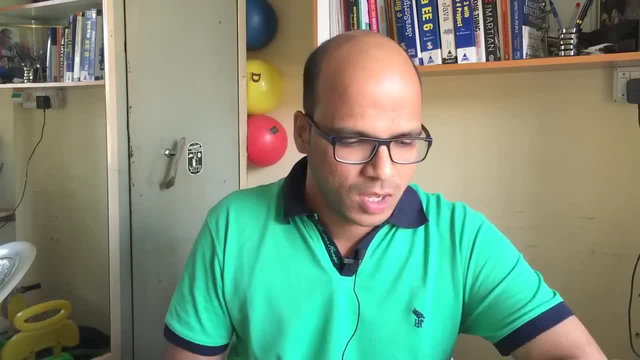 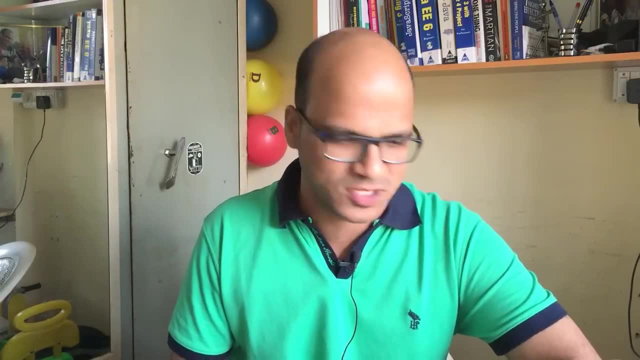 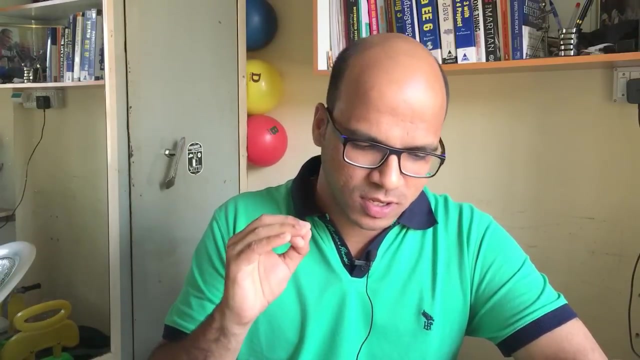 have boilerplate codes and it is concurrent. now, what else? in fact? there is a quote you know from, from one of the famous person, so let me just quote it. so the quote is from Alan J Pallis, and he says a language which, so a language that doesn't change the way. 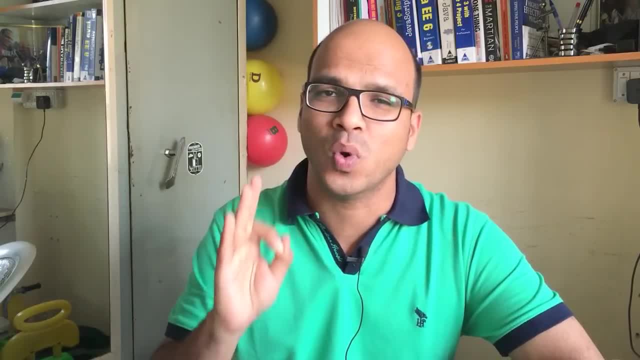 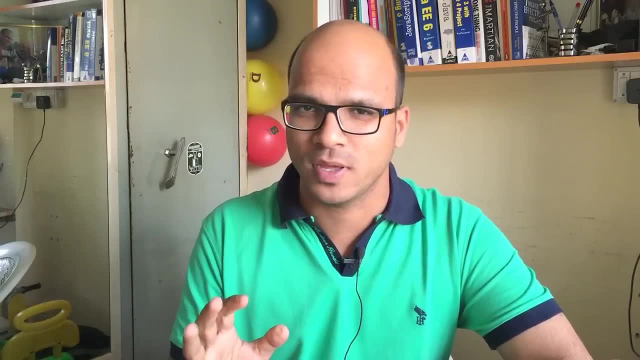 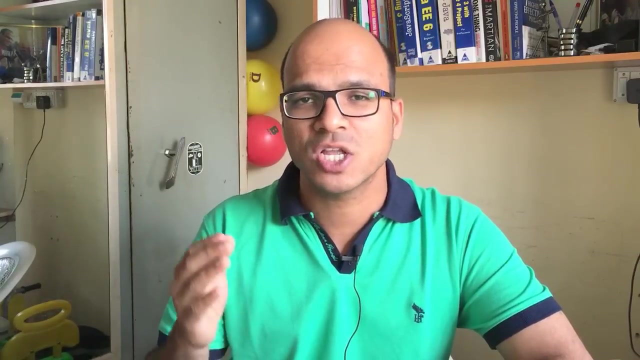 you think about programming is not worth learning. so that means after a language is learning, so that means after learning Scala. it will change the way you think about programming. no, it's not more about procedures, it's not about objects. now it's more about functions. because Java is functional, sorry. Scala is functional programming. sorry for that Java. 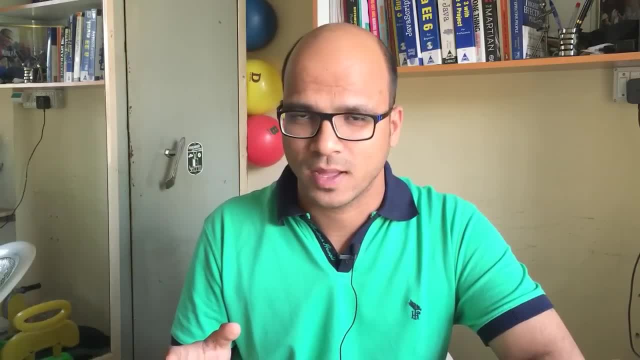 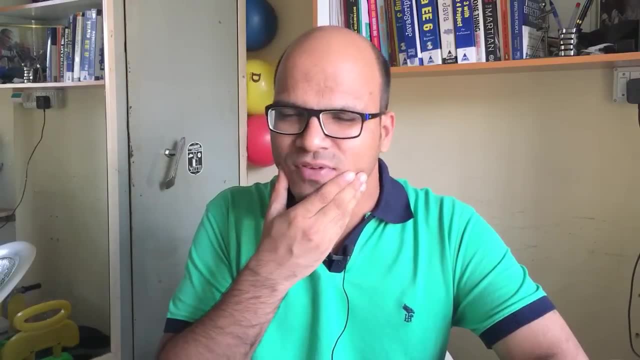 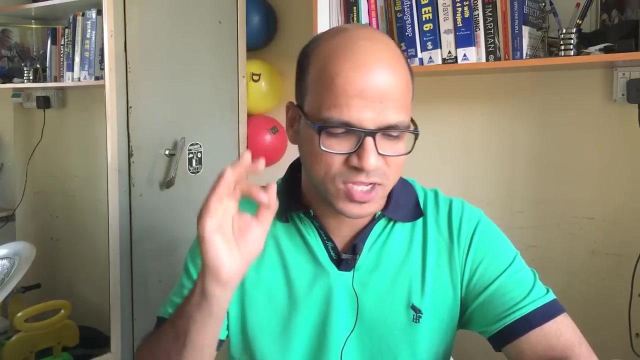 part. so Scala is a functional programming. ok, so in Scala we have to focus only on functions. so if Scala is functional, then other language is not functional. I don't know. so Scala is, but Scala is functional programming. so again, let me repeat that quote: a language that doesn't 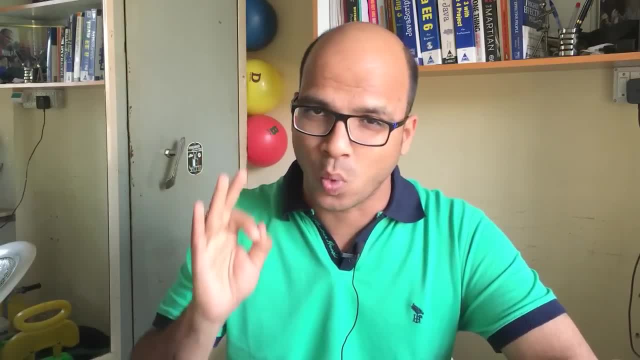 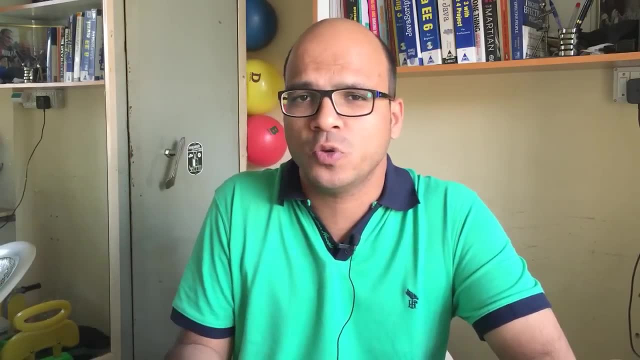 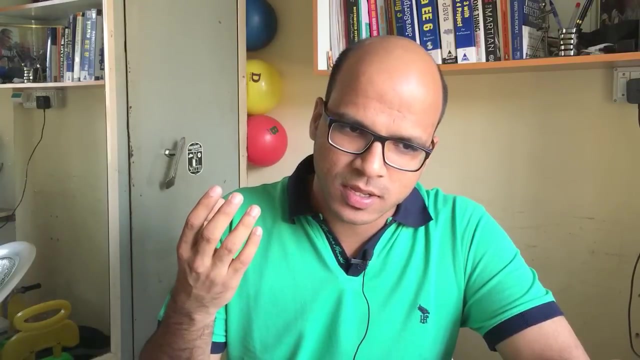 change the way you think about programming is not worth learning and trust me, after learning Scala, it will change the way you program. now it may happen that you don't want to make your career in big data, you don't want to do any other stuff, but it's even if you learn. 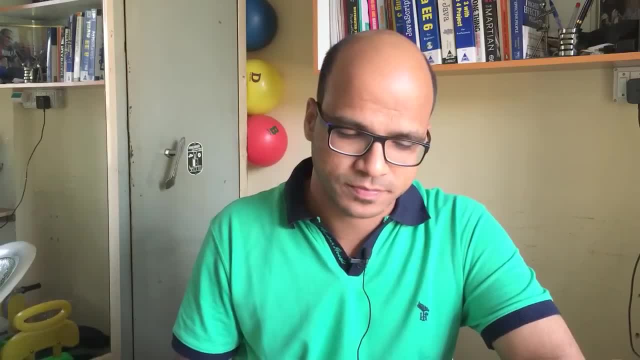 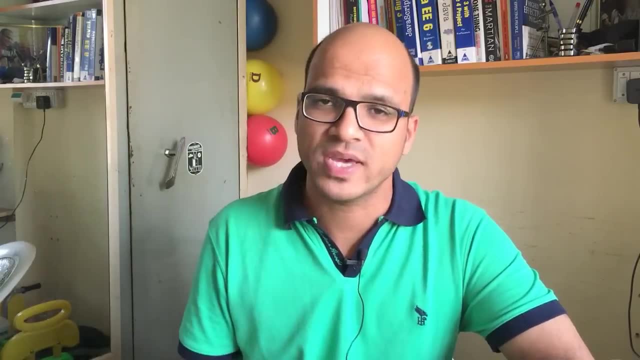 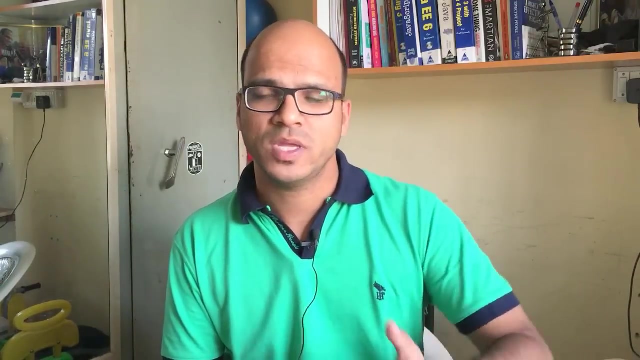 Scala. it will change the way you write your Java codes. now what else Scala is faster than Ruby, Python, Nodejs, Java itself. so Scala is faster than all these languages. now people are going for Python, they are going for Nodejs, but, trust me, none of these languages are faster. 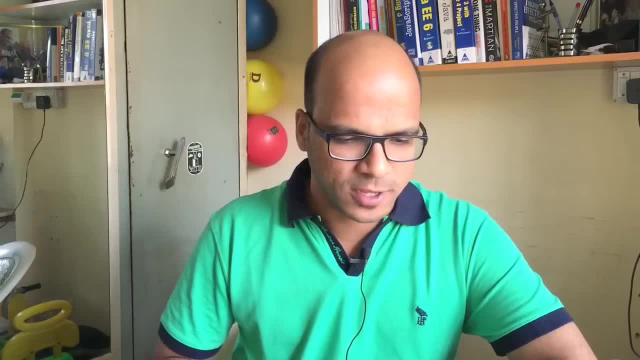 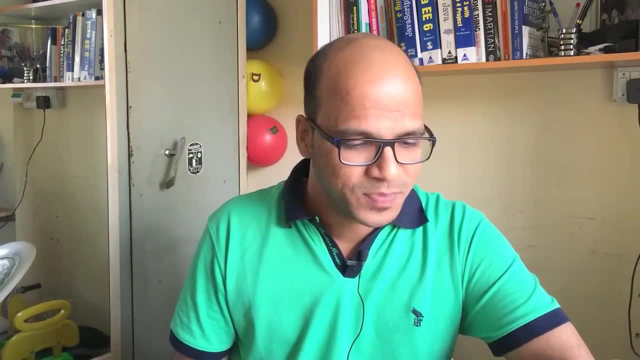 compared to Scala. ok, so that's that's one thing and one more reason why to learn Scala. so, even if you are a Java programmer and if you want to learn Scala, the reason is, if you are a Java programmer and you want to spend more time with your family and friends, you 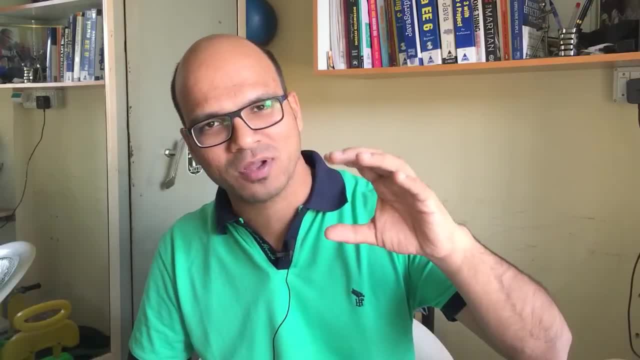 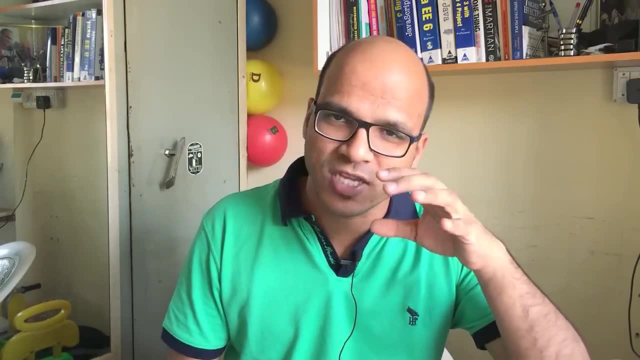 should learn Scala, because that's the. so if you want to do a particular task in Java in between 20 lines, you can do the same stuff in Scala in 5 to 6 lines. so you don't have to waste- I mean, you don't have to waste your much of time in writing that code. second advantage: 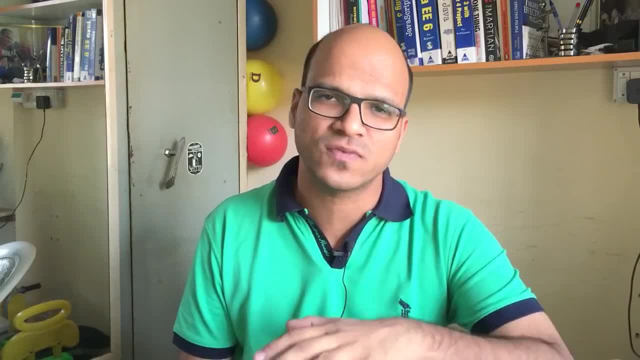 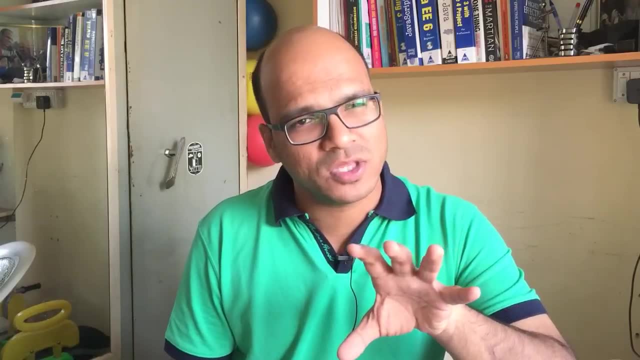 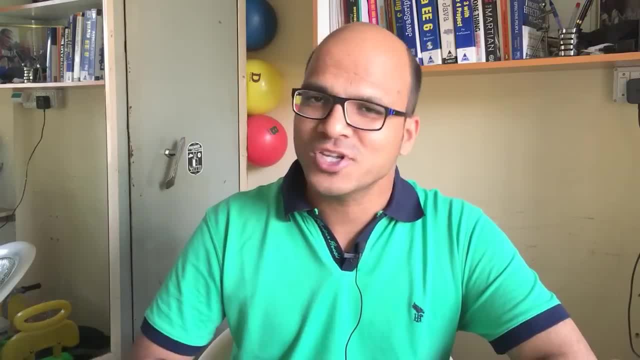 that bug is, and Scala is very you know your code in Scala looks beautiful. so even if you have a bug, it is difficult to detect where that bug is, and Scala is very you know your. Now question arises: should you leave Java and learn Scala? That means that's the end of Java? And the answer is no. Java will be there forever, But there are certain requirements where Scala works much better than Java. Example: three years back, I mean when Twitter was made in 2009,, I guess. 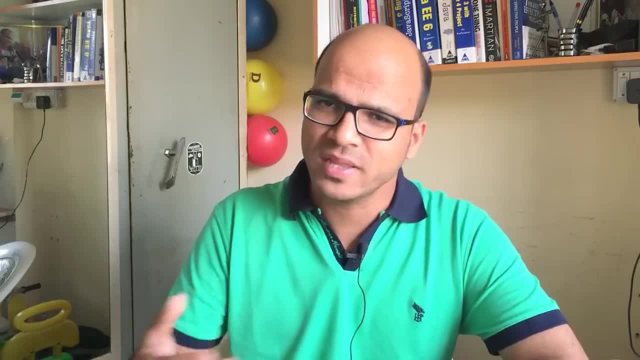 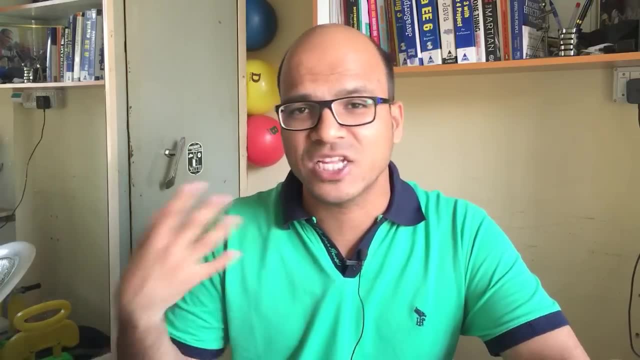 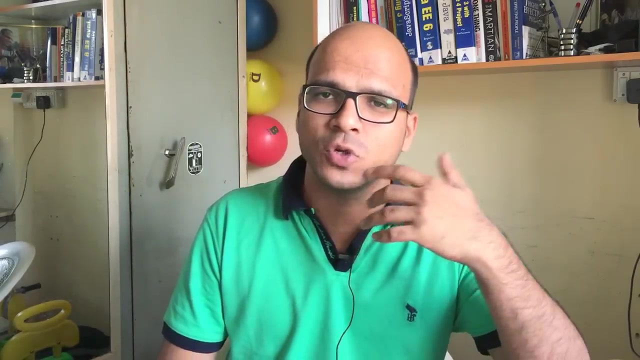 they used Rubio language to make Twitter, But later on, you know, because of lots of tweets, because of this big data concept, because of elections, because in elections, you know, there are lots of people, they tweet on Twitter. So it was very difficult for Twitter people to manage all this data using Ruby language. 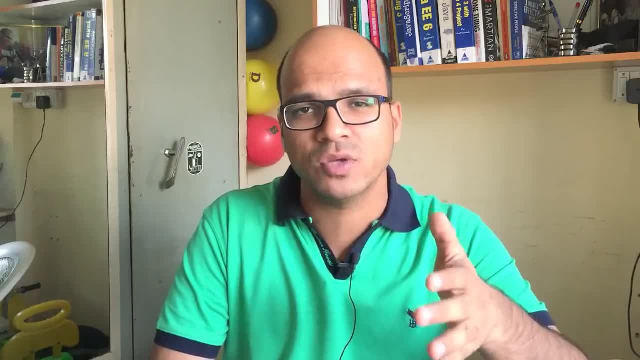 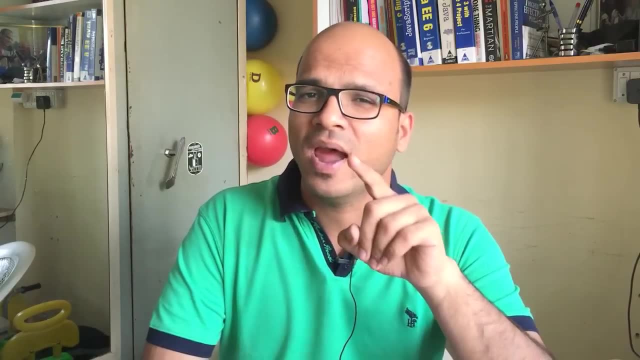 So what they did? they removed the Ruby from the backend and now they are using Java and Scala for the backend. That means they are using both Java and Scala. That means they work together? and the answer is yes, Java and Scala they work together. 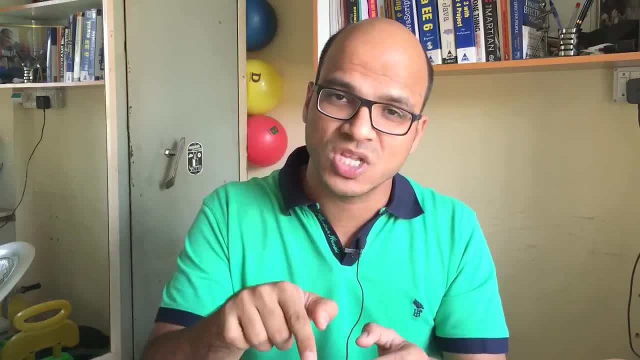 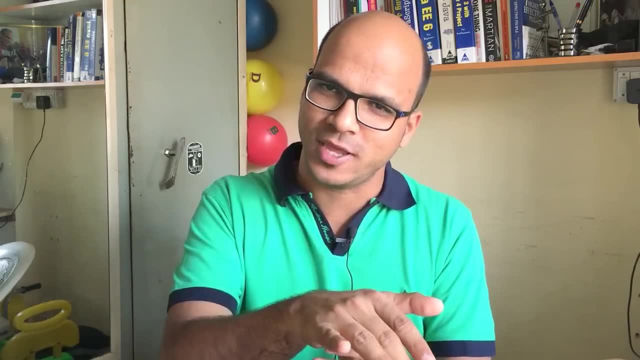 It's because Java runs on JVM. even Scala runs on JVM. That means you can run. you can write one application which is Java based application, and you can. you are using Scala code there And you can make a Scala project in which you can run. you can write Java code. 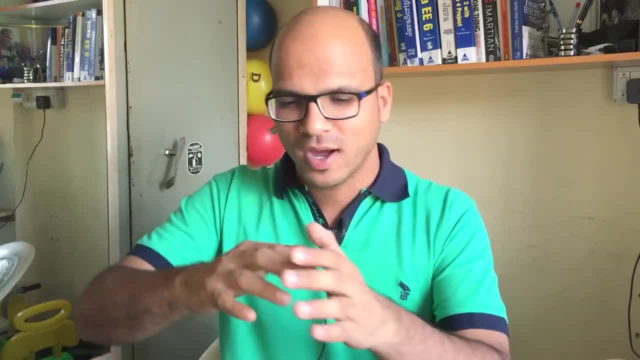 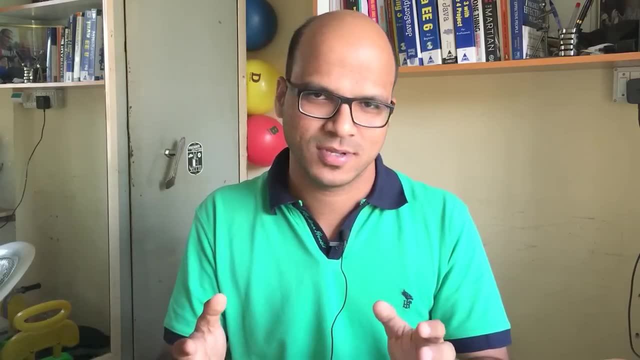 So that means a Java project supports Scala code, a Scala project supports Java code. So in Scala we can use all the Java libraries. Okay, So if you know, So if you know Java, you can learn Scala in one month. 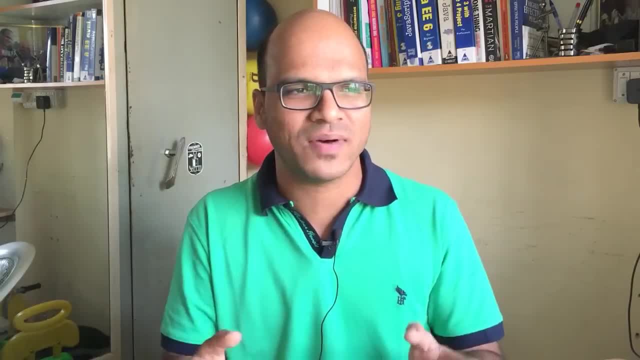 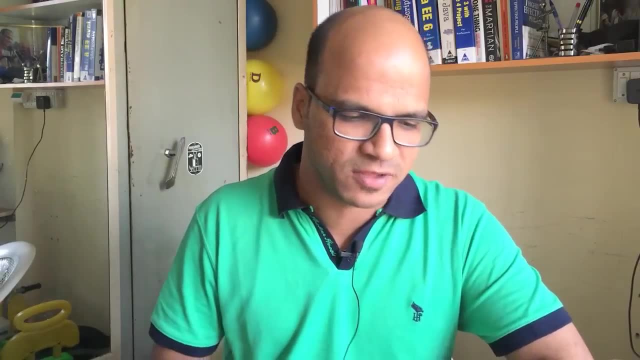 It is that simple, provided you know Java. If you don't know Java, then Scala. yes, it is a bit difficult to understand. I am not saying it is impossible to learn Scala if you don't know Java, but it is. yes, it is a bit difficult to understand. 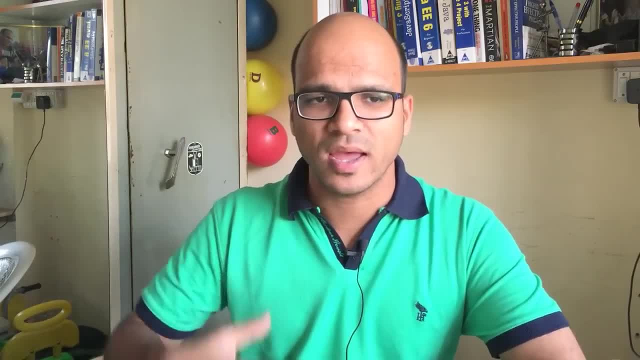 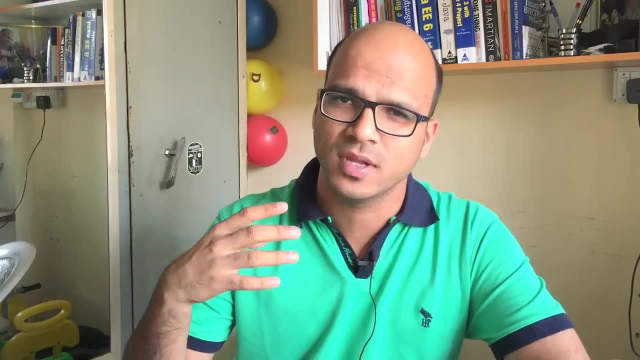 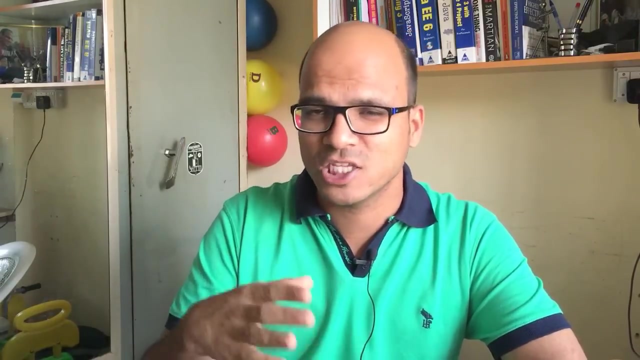 What else? That's it. So Scala and Java works together. Okay, So Java and Scala works together. So if you write: So Scala works on JVM and nobody loves Java, Okay, Everyone loves JVM And Scala is powerful than Java. 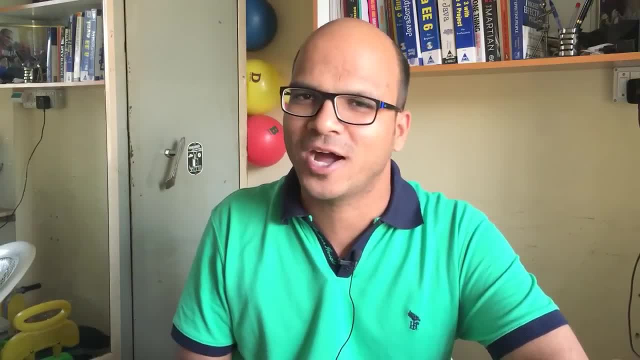 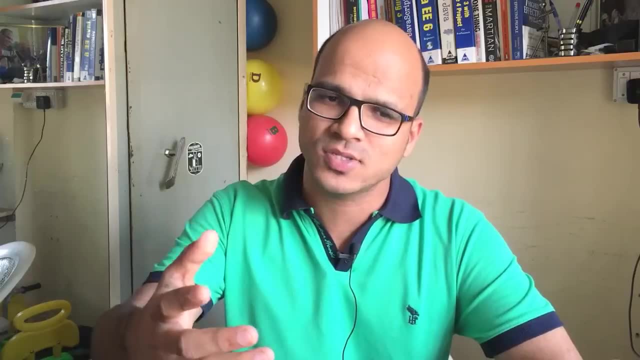 So Scala works on JVM, So we love Scala. So in the next video we will talk about the setup of Scala and how to write your first code. So let me know your thoughts about Scala so that we can continue. And if you have not subscribed the channel, please do it. 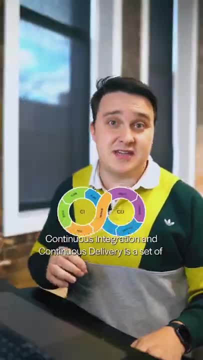 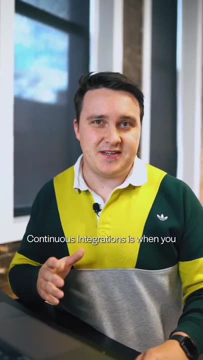 What is CI-CD and do I need it? Continuous integration and continuous delivery is a set of DevOps best practices when merging and deploying your code. Continuous integration is when you merge your code into a repository and you want to do things like check the quality.